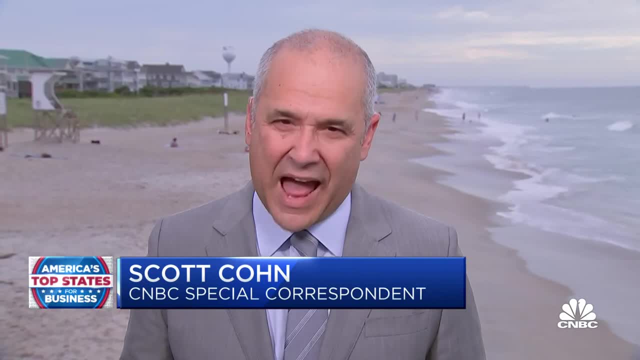 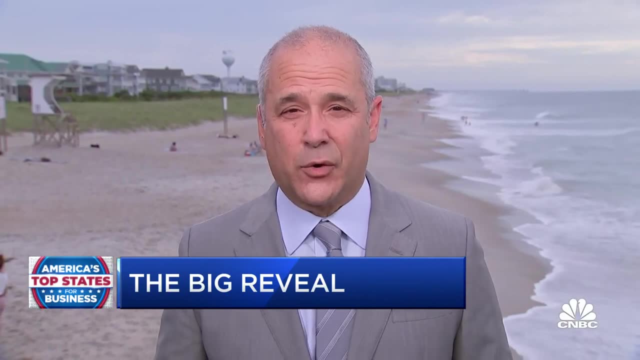 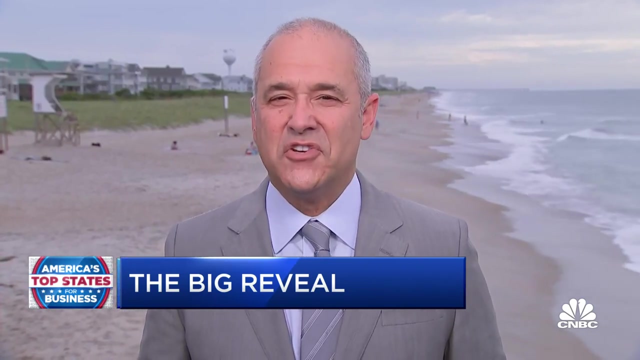 The mystery will be a mystery for not too much longer, Andrew. We go through all 50 states, 88 metrics in 10 categories of competitiveness, to find out which state is America's top state for business. Ladies and gentlemen, start your engines. Hey, I'm Dylan Hart Jr and I know a. 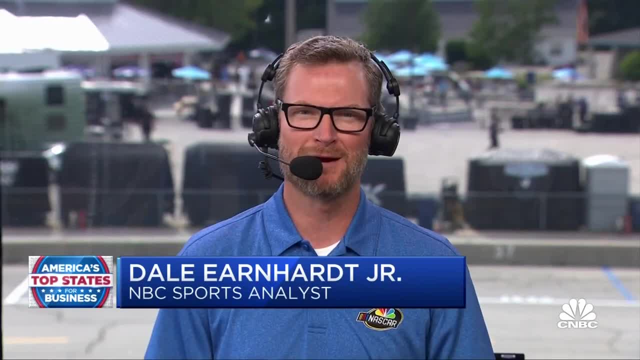 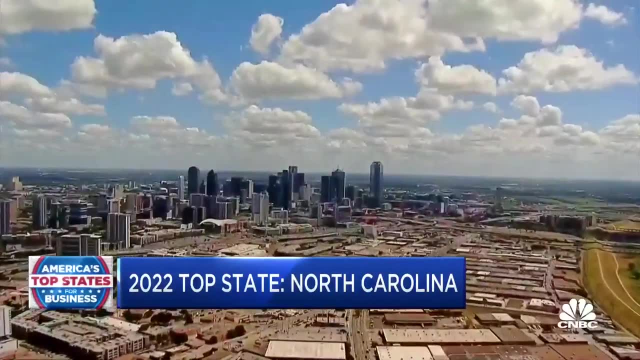 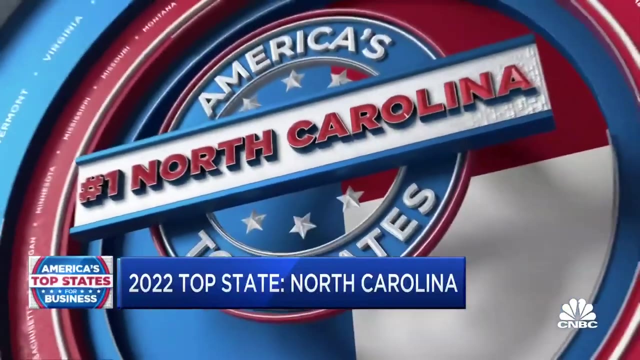 thing or two about finishing first, and my home state of North Carolina is America's top state for business. Our 50-state journey puts every state to the test. This year, the winner stands clear: North Carolina, the Tar Heel state, with 1,580 out of 2,500 points- America's strongest. 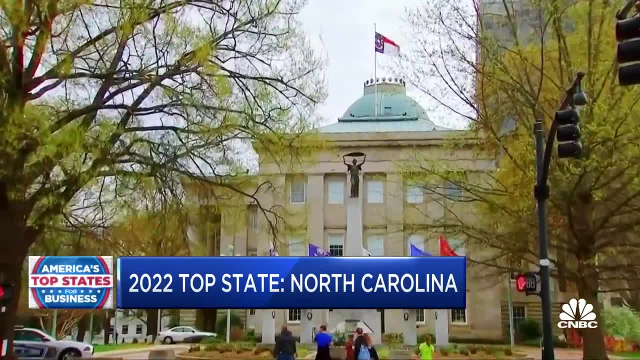 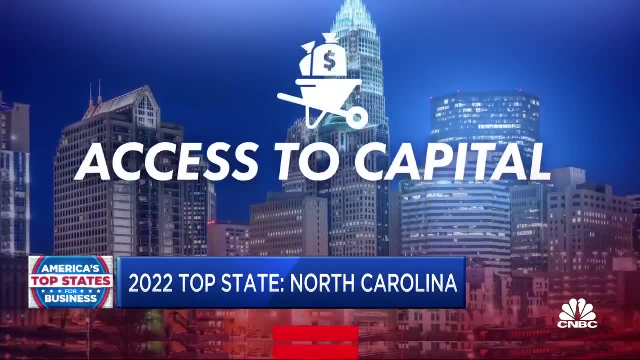 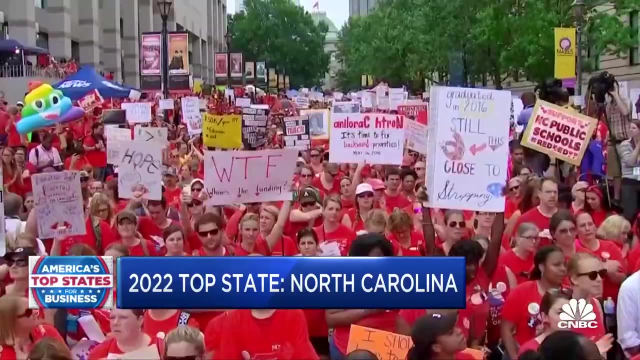 overall economy. according to our study, with strong state finances and a solid housing market, This banking hub second only to California in access to capital and in the top five for technology and innovation In a divided country, the divisions in North Carolina are deep. 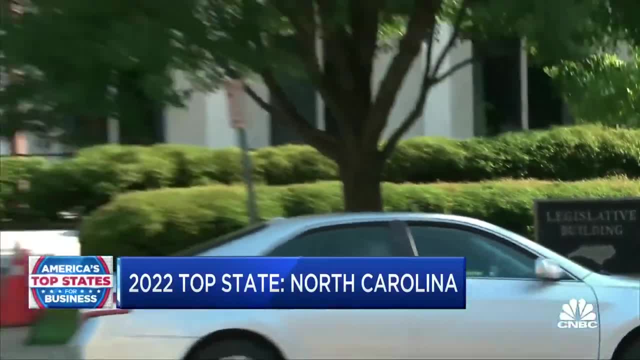 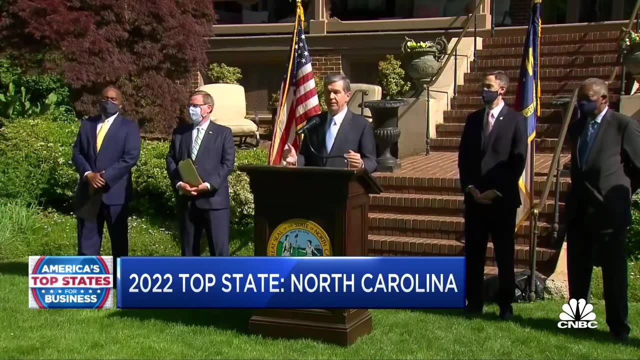 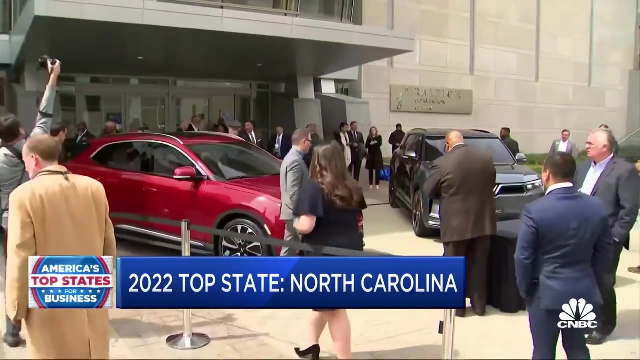 But Democrats and Republicans keep managing to put them aside to win business. Apple's first corporate campus on the East Coast announced last year And this year a $4 billion investment promised by electric car maker VinFast. I'm very proud to call North Carolina my second home. 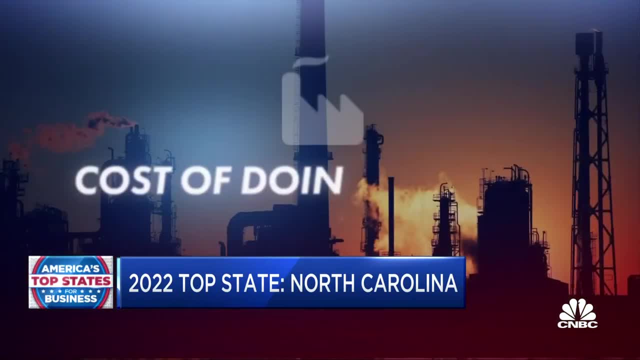 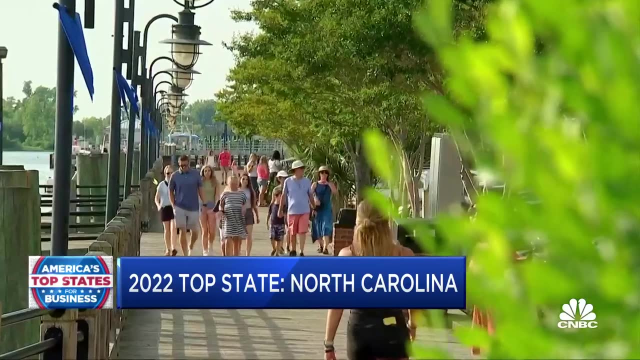 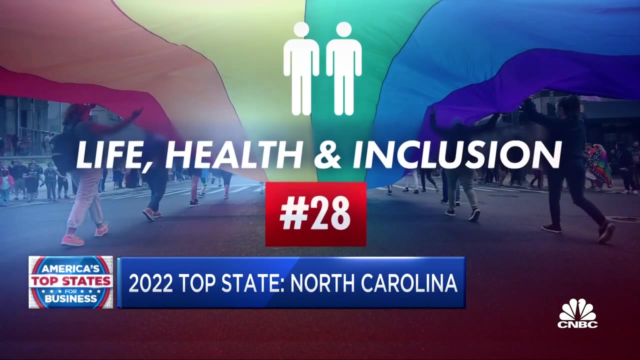 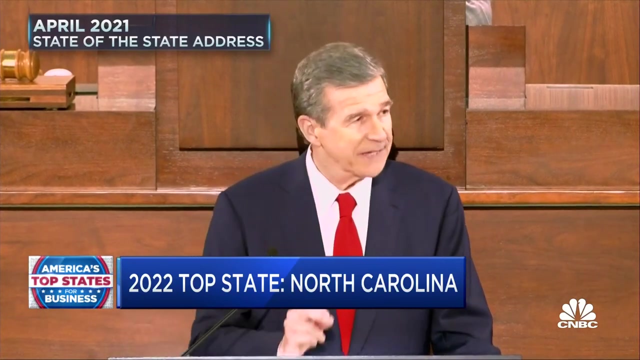 But this state has growing pains. They're raising the cost of doing business, Health care resources like hospital beds and public health spending aren't keeping up And with no statewide anti-discrimination protections, North Carolina finishes in the bottom half for life, health and inclusion. We must confront systems that favor some and harm others, and we must fix. 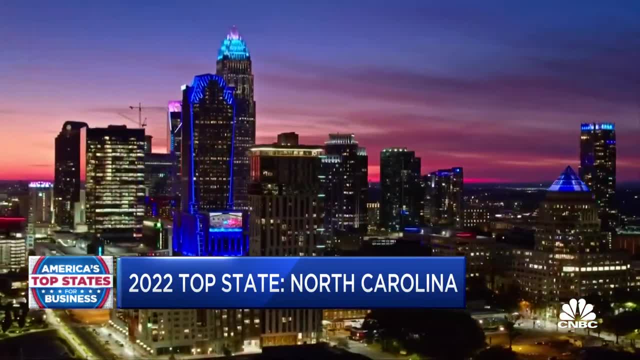 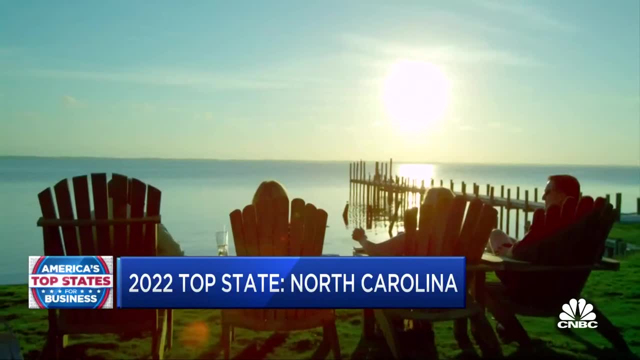 them. For as long as we've been rating the states, this state's been a contender, but never number one. until now. From the Smoky Mountains to the Albuquerque Mountains, the state's been a contender. out of a thousand state-owned businesses, The state has raised $1.1 billion for its national 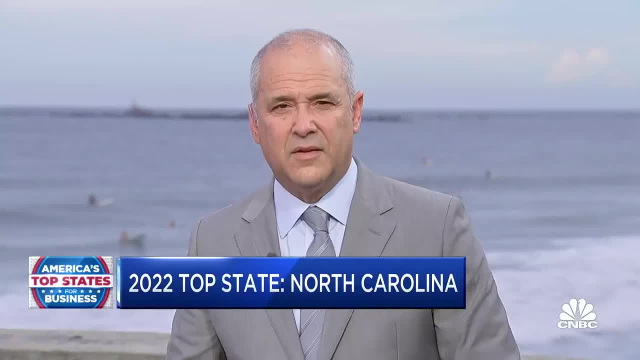 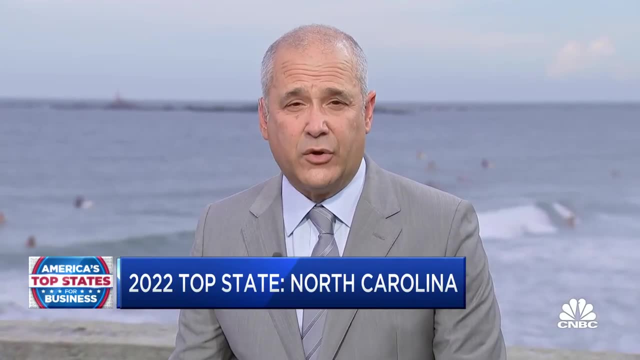 business and has been one of the biggest in the history of the United States segment of American History. it's all due to the four best states in the world, Outer banks and the big banks. North Carolina, America's top state for business 2022.. 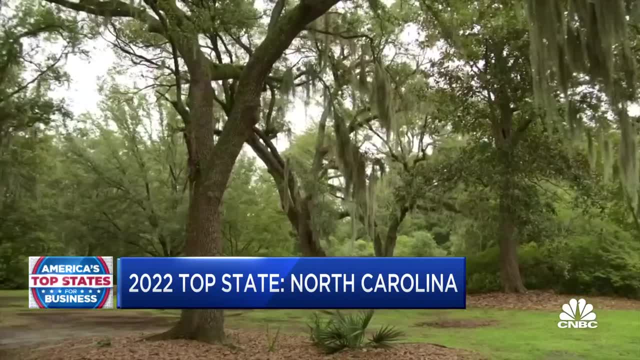 Where were we yesterday? Yesterday we were at Air Lee Gardens, not far from here in Wilmington. It is on land that was deeded to local families In 1735 by king George II. New Hanover County purchased the site, or. 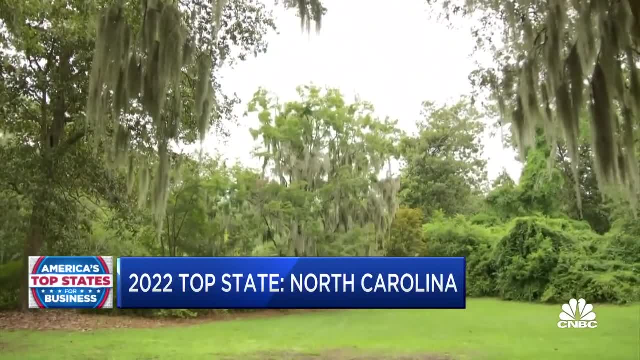 portion of the site in 1999, and turned it into a beautiful public park. Now here's the State's Law Enlargement in our state. there's a lot to do In some states. it's one of the most Now about those hints that you've been guessing so well over the last couple of days. 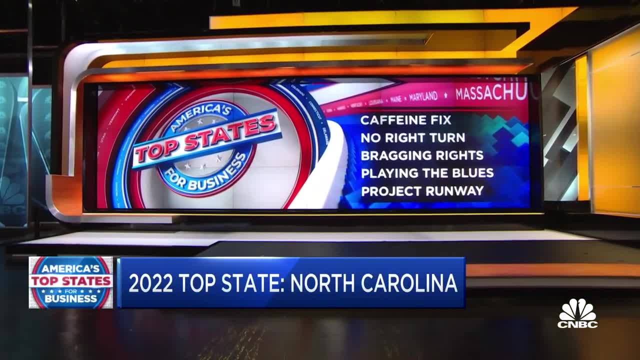 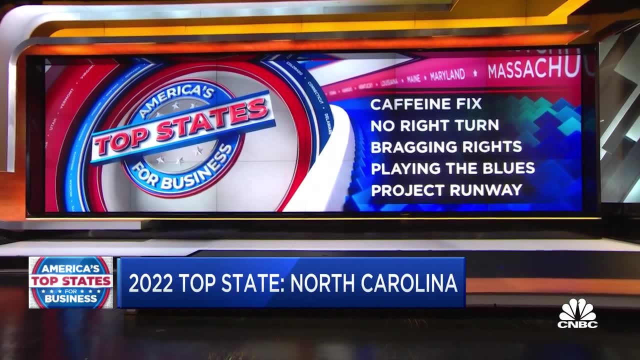 Caffeine fix. Yes, Pepsi-Cola was introduced in New Bern, North Carolina, originally called Brad's Drink, in 1893. And a 12-ounce Pepsi has about 5 milligrams more caffeine than a regular Coke. There's your caffeine fix. 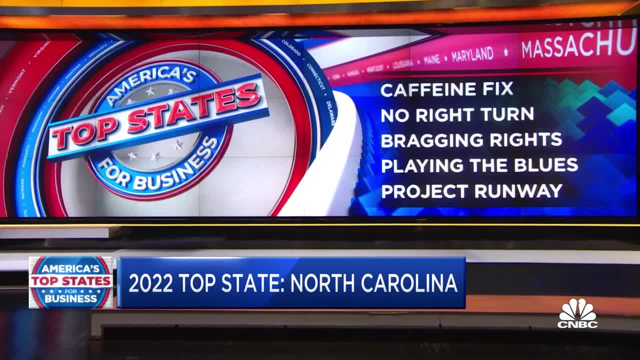 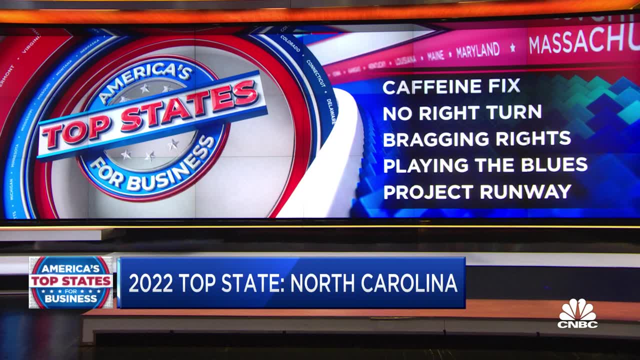 No right turn. A lot of people got this. The first NASCAR Strictly stock race was in Charlotte in 1949. The standard NASCAR track runs counterclockwise, So no right turns. Bragg and Wright's largest US military base is Fort Bragg, west of Fayetteville. playing the Blues. 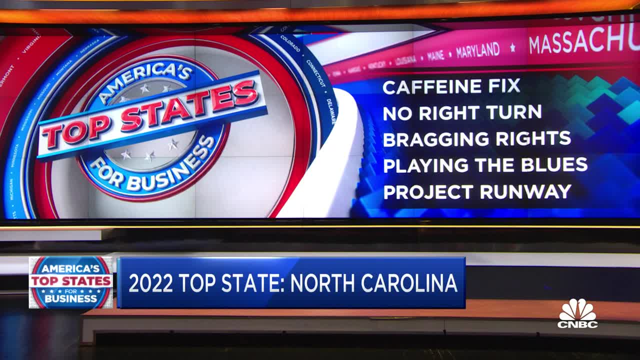 Those are the colors of the Duke Blue Devils and the North Carolina Tar Heels Project Runway. the first powered flight not far from here, Kill Devil Hills, near Kitty Hawk, North Carolina, achieved by the Wright brothers in 1903.. 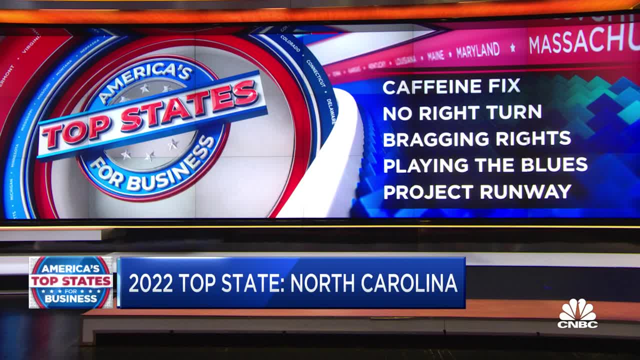 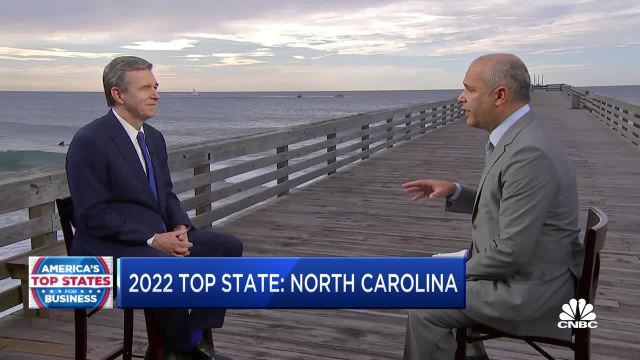 Roy Cooper is the 75th governor of the state of North Carolina. North Carolina has been in the top 10, 13 of the 14 previous years, but never number one Until now. congratulations on that. How do you think you did it? 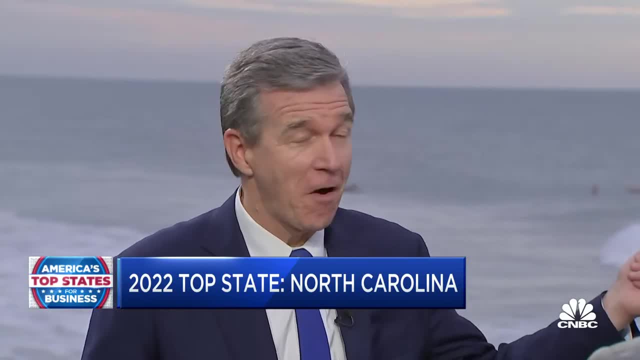 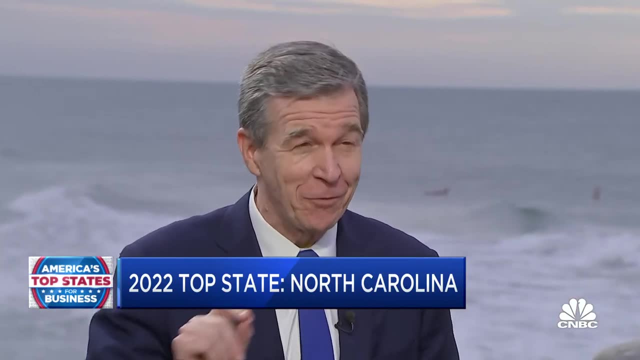 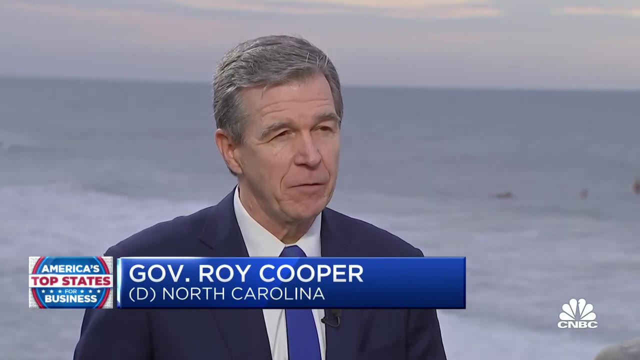 Well, one thing, it's just the people of this state. I hope you saw that beautiful North Carolina sun rising over the ocean this morning And, by the way, PepsiCo is still incorporated in North Carolina, not Delaware, But we've pulled together in a bipartisan way to make sure that businesses know that we've got. 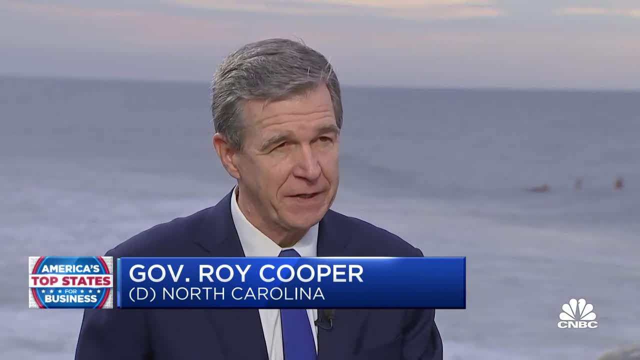 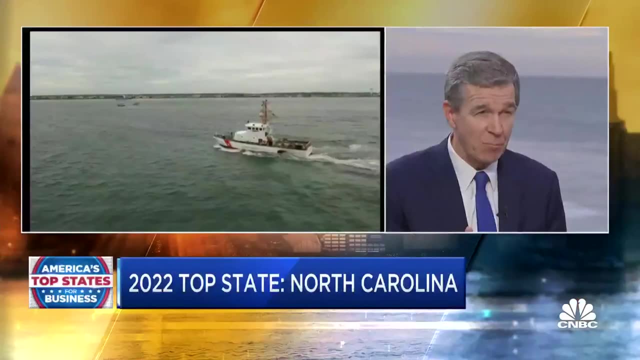 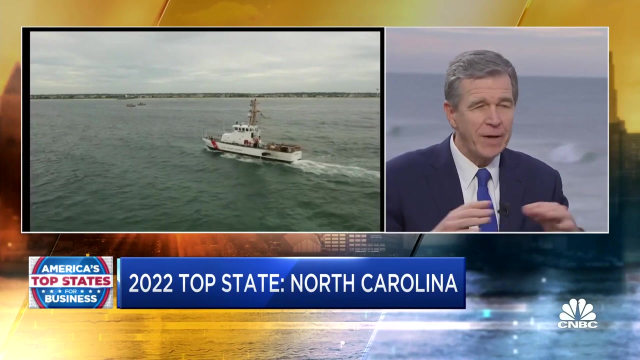 the most talented, educated workforce in the country And, talking to CEO after CEO, The workforce is the driving force for them right now And they see North Carolina as a place where they can rely on our community colleges, our greatest array of private and public universities in the country. 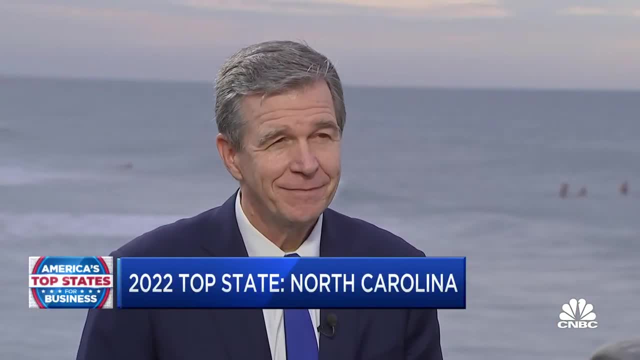 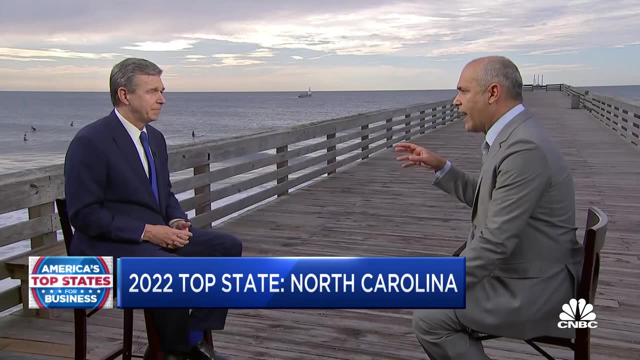 to make sure that they have the workforce that they need. You mentioned at the top of this bipartisanship And I'll tell you, it's interesting. We go through all these numbers and we get to the top state and then you start to look around. 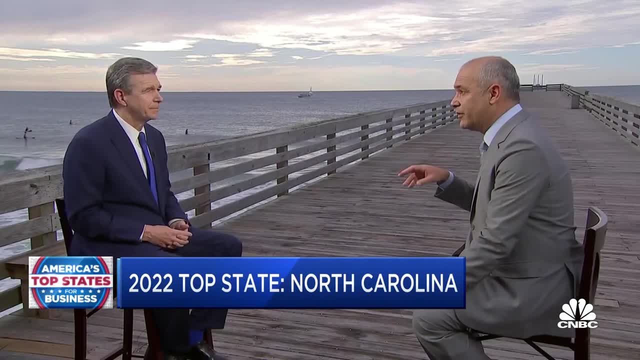 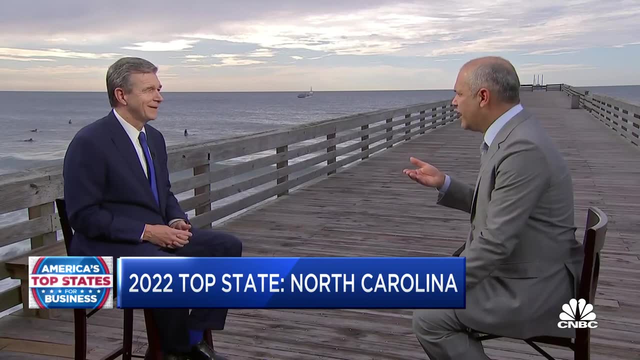 And what you're achieving here in terms of bipartisanship, the Republican generalist Assembly and you- I guess you guys didn't get the memo about how you're not supposed to cooperate, but tell me how that's worked. You didn't come in with that kind of relationship with your. 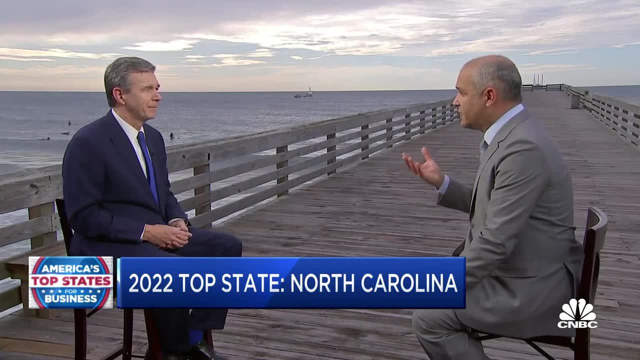 Republican colleagues. You have it now. We have this potential, very real potential, that it's divided government federally next year. How have you done it here and what's the lesson? Is there a lesson for the country? Well, first, we disagree about plenty. 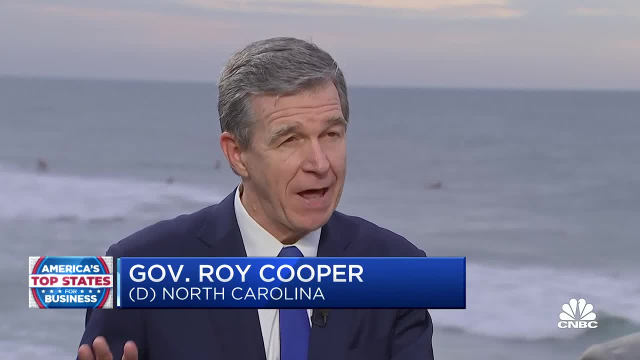 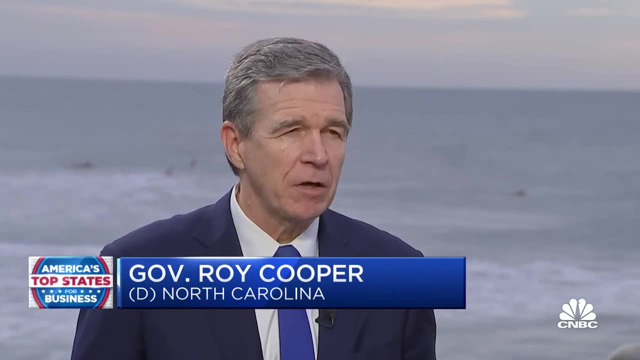 and my vetoes have been able to stop a lot of bad legislation that's come forward, particularly in the cultural wars. We've been able to keep that at bay. But I think we all agree that high-paying jobs for our people is something we have to agree upon. 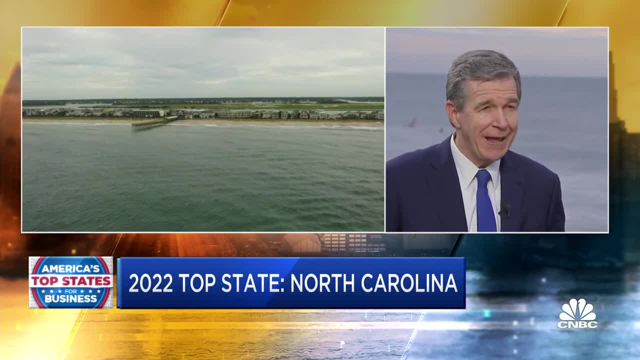 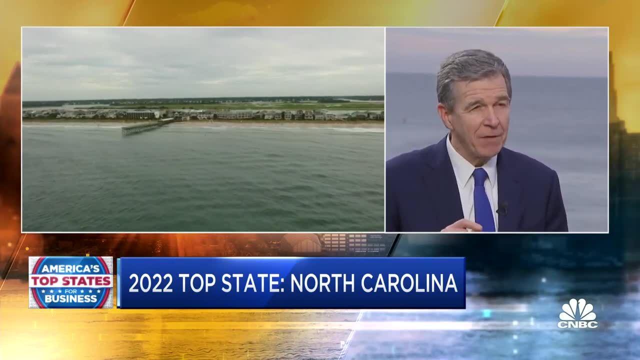 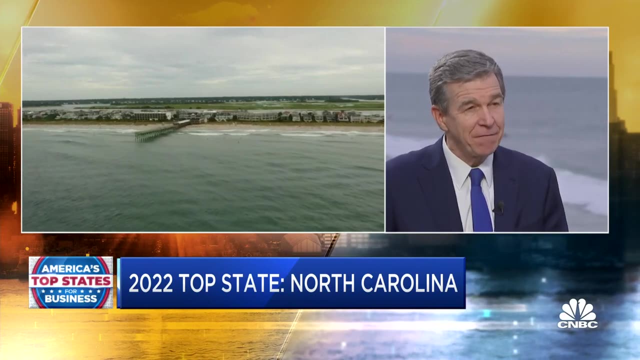 and this General Assembly has trusted my administration and me to go out and negotiate deals. We don't have the greatest incentives across the country, but we have enough performance-based incentives that put us at the table Where we can show our wares. they provided the funding to do that with our job development. 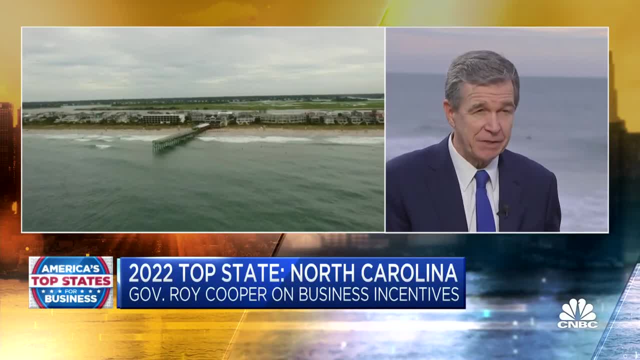 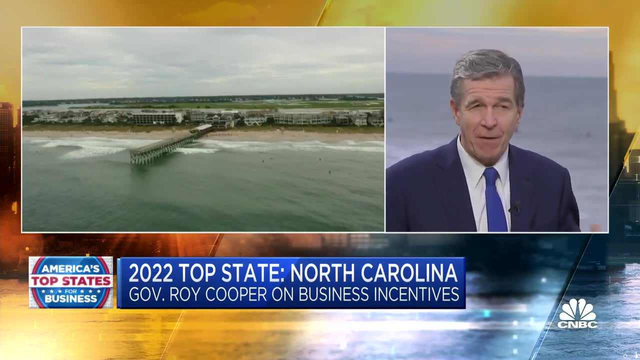 incentive grants, the help with infrastructure that businesses are looking for, the extra help with job training that they may need in a specialized way. We've worked together. I know that we've met with CEOs and I've had both Republican and Democratic leaders of both the. 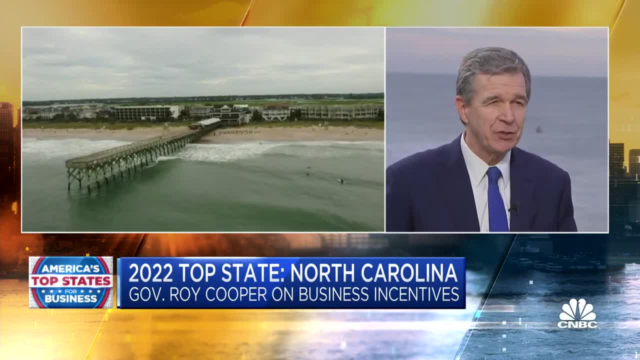 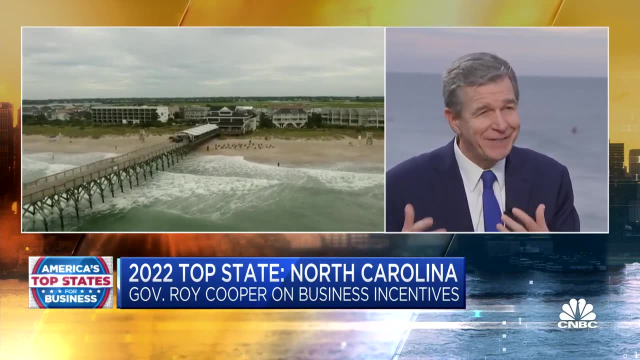 House and the Senate on each side of me as we make a presentation to the company that this is where you need to be. You're going to get predictability, Reliability, consistency. Businesses look for that and they also look at what happens after the. 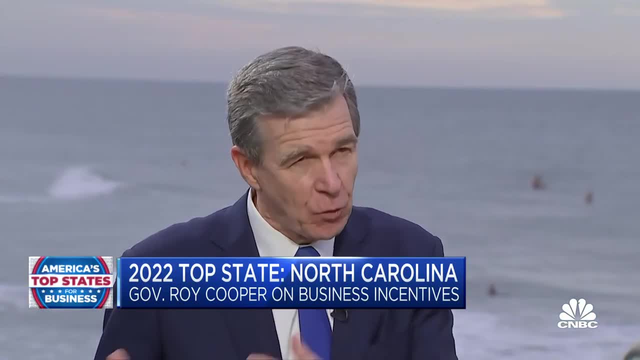 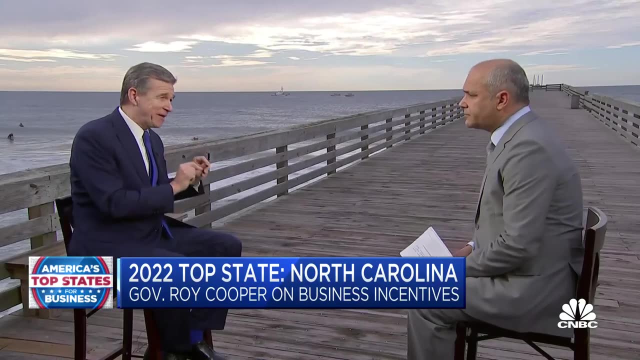 deal is done, Does state government, local government, continue to work with them and try to help them succeed? Some of our best recruiters are CEOs that are already here and know the North Carolina story. I want to ask you about some of those deals, because one of the things that you've 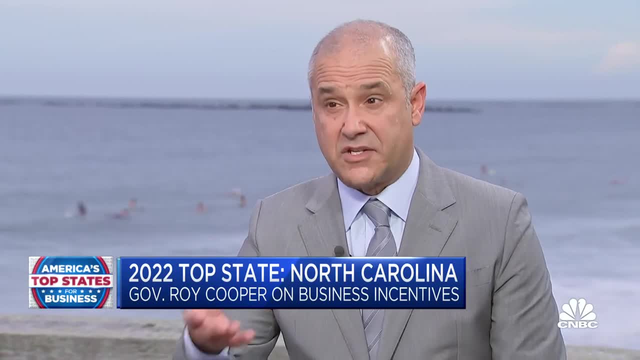 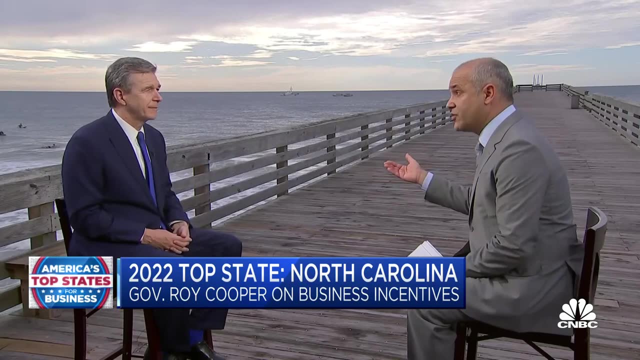 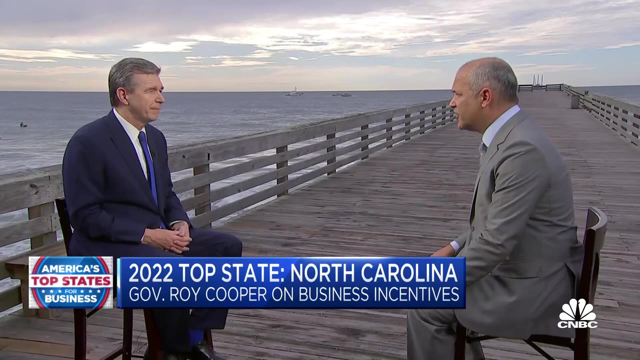 been able to achieve with this bipartisanship is higher incentives and there's some pretty common ones. This deal with VinFast, which is a new company unproven in the electric vehicle market in this country. that's some healthy money- $1.2 billion, I mean. how do we know? how do the 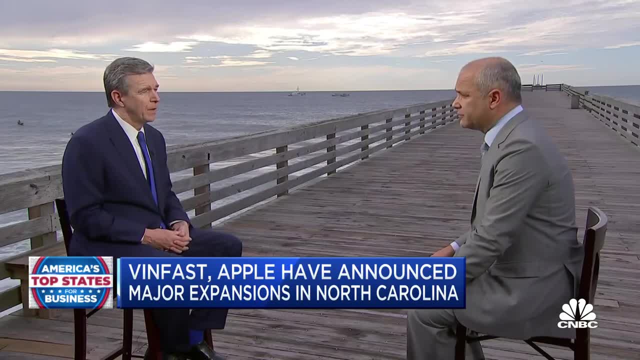 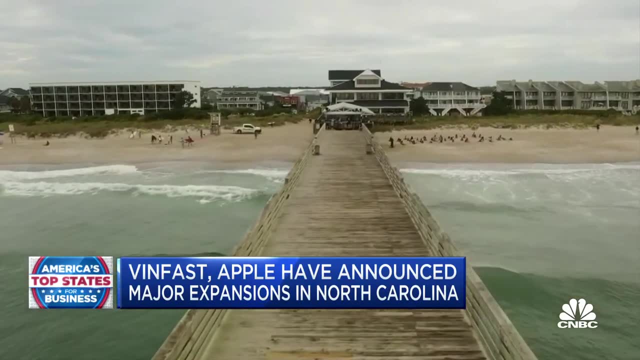 taxpayers here know that they're going to get their monies right. First we do a detailed analysis to predict what kind of income will come to our state, how much we will benefit. If it is a significant net positive, then we'll do it. 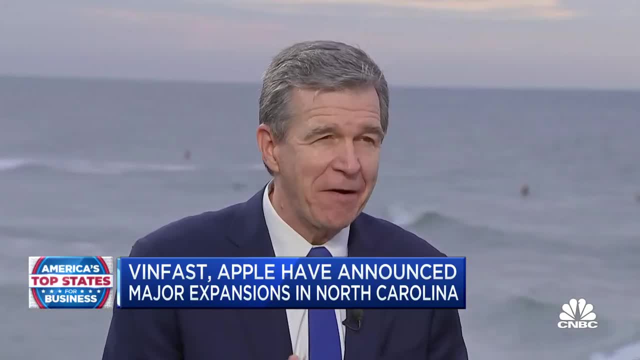 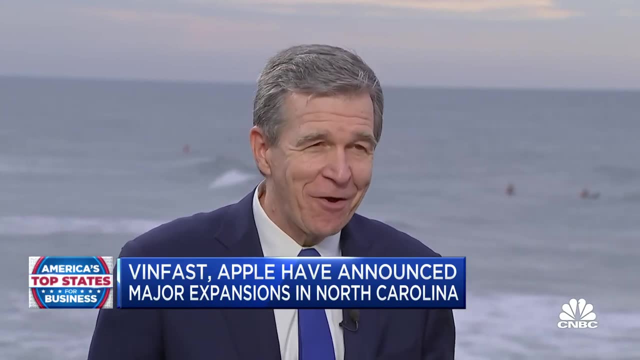 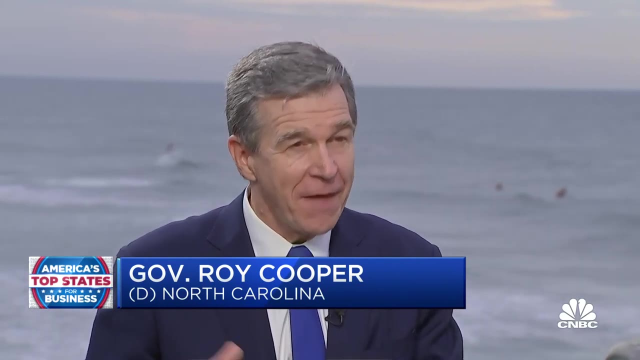 There have been a number of deals where it just didn't meet our analysis. With VinFast we're on the cutting edge of the clean energy economy. You know we've been trying to get auto manufacturing for a long time in our state. We now have it at the time where EVs are there and are coming fast and we 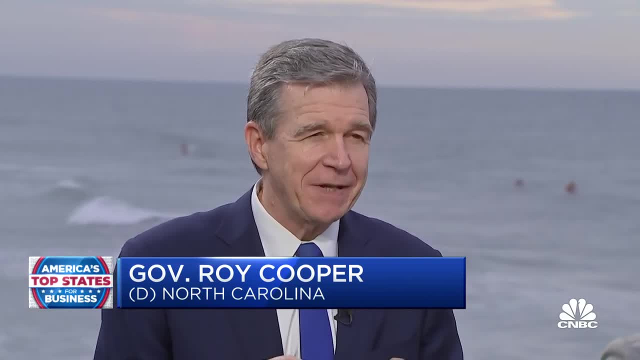 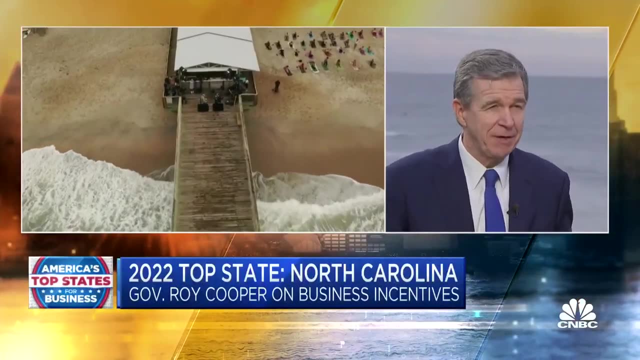 want to be on the cutting edge, But ours are performance-based. They have to create the jobs at the salaries they say they're going to create them in order to be able to do that. So we're trying to get the tax benefit. The other funding comes in for infrastructure, roads, water and 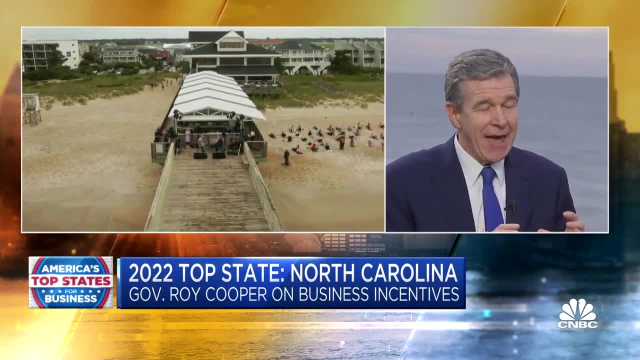 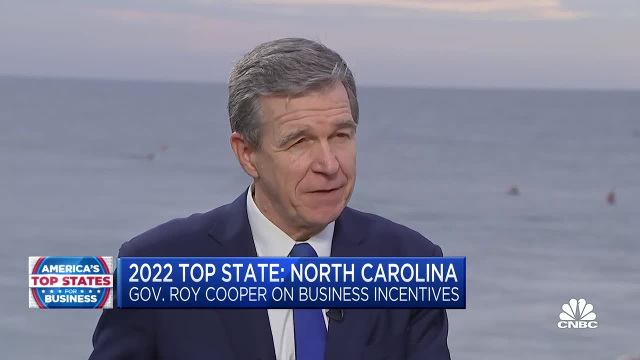 sewer, things that you need anyway. We've had mega sites that have been extraordinarily successful in attracting businesses to our state. In this last budget that I signed, there's more investment to develop more, because we're running out of them, because we have so many businesses that are. 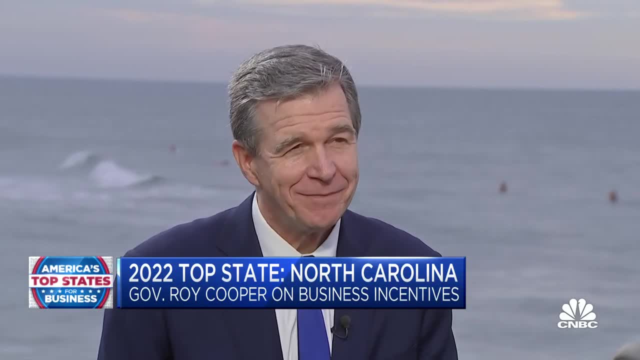 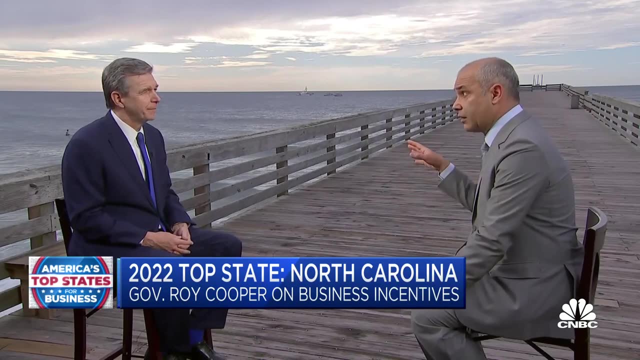 interested in coming to North Carolina and expanding here. I want to ask you about the weaknesses that we found. a couple of them. One is the fact that the costs are going up. They're going up everywhere, but North Carolina's costs are going up. 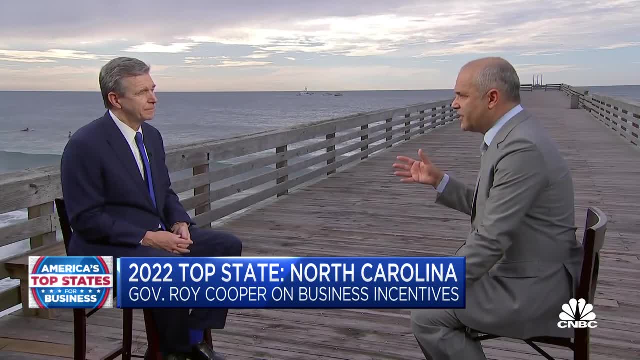 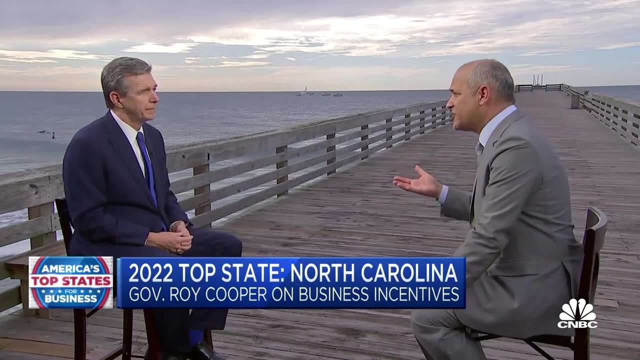 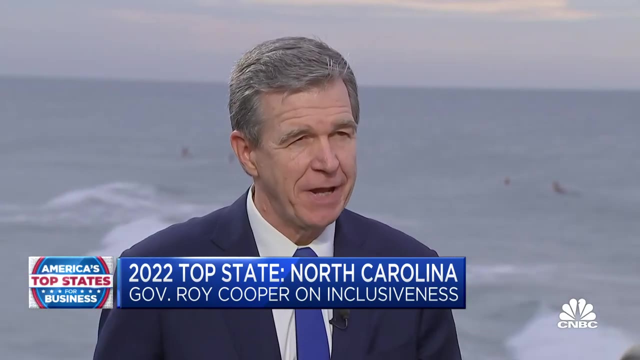 probably growing pains, And also this issue of inclusiveness. It's something that's been you've been dealing with since you came into office. There is no statewide public accommodation law. Is that going to change? So, number one, I've appointed by far the most diverse cabinet in the history of our state. 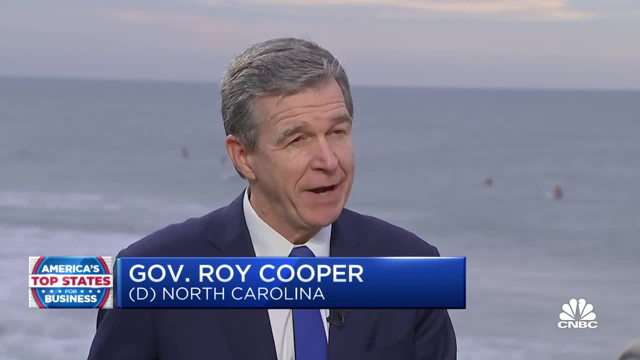 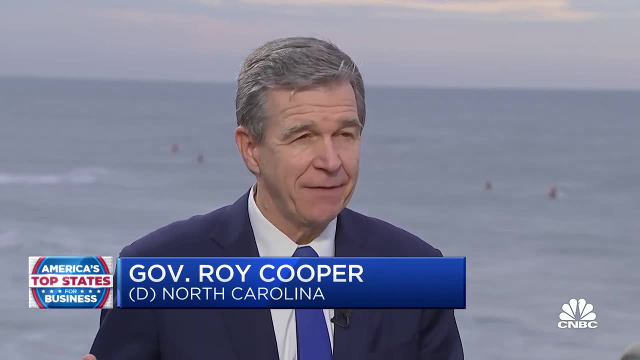 We are number one in the country for the percentage of women in our tech workforce. We have more four-year HBCUs than any state in the country, And North Carolina A&T State University graduates more black engineers than any state in the country. 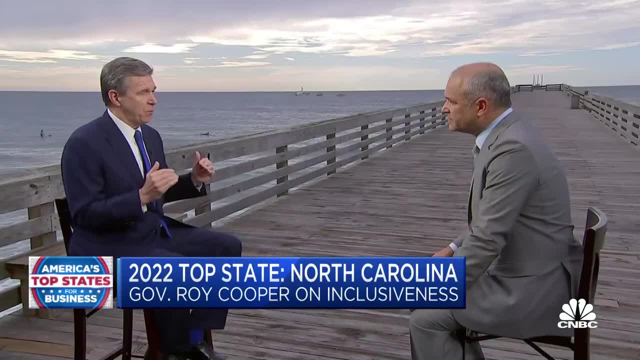 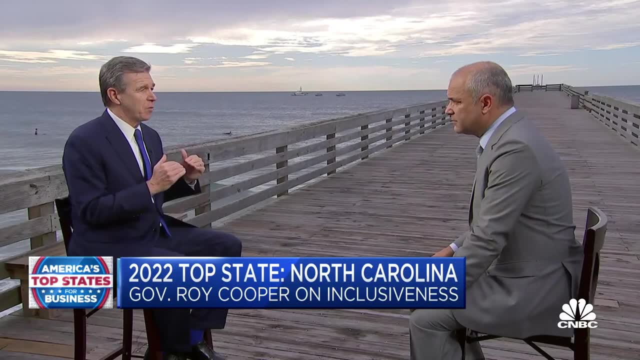 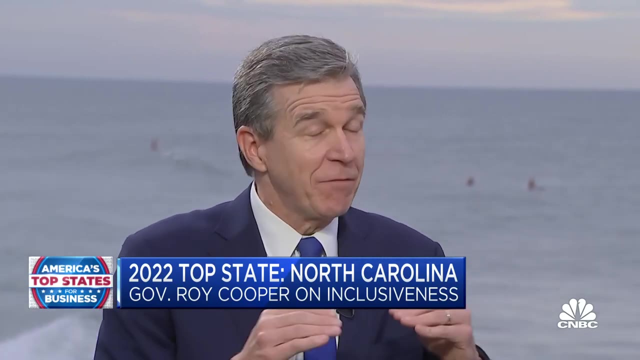 But you don't have the protections in state law. Well, I've issued executive orders to make sure that we are protecting our LGBTQ plus community. I've issued an order banning any contracts with organizations that engage in conversion therapy. We have repealed the horrible. 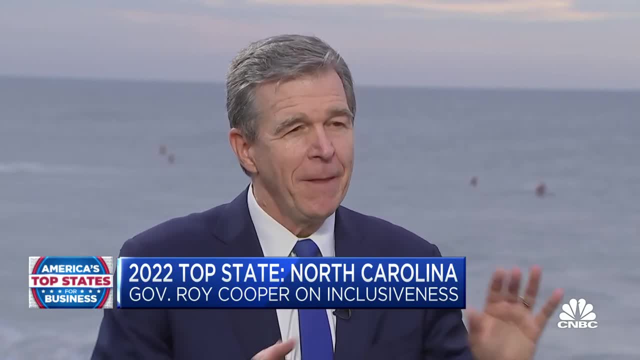 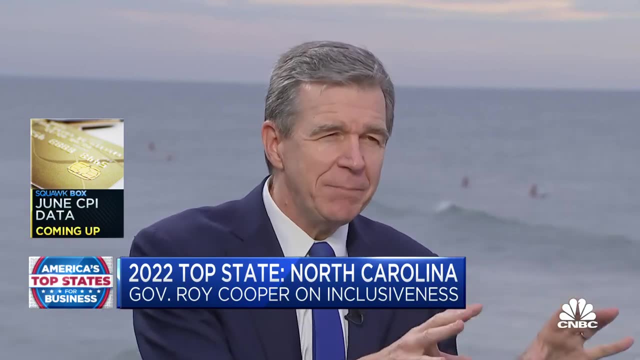 Bill 2 bathroom bill completely in North Carolina. Now we're holding them at bay on the culture wars, But I think they have come to the realization that we don't need to be doing that. Not only is it the wrong thing to do. we may disagree on whether it's the wrong thing to do. 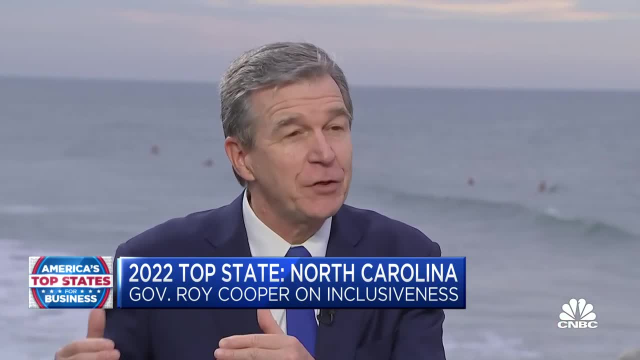 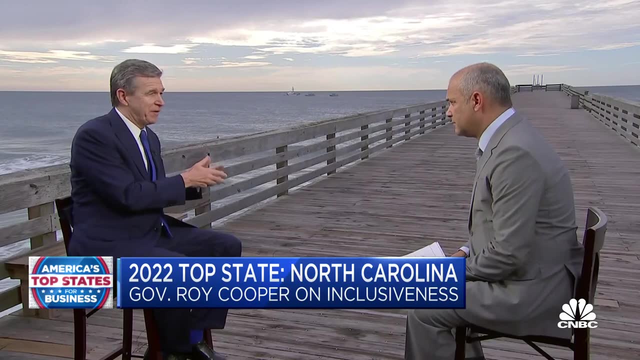 I think it is, But we know that it's good for business. For example, you know we're on the other end. There's a business in Arkansas putting together a film, producing a film, Arkansas's abortion ban goes into place. 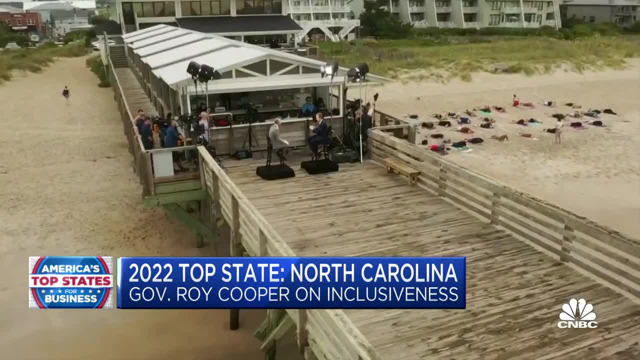 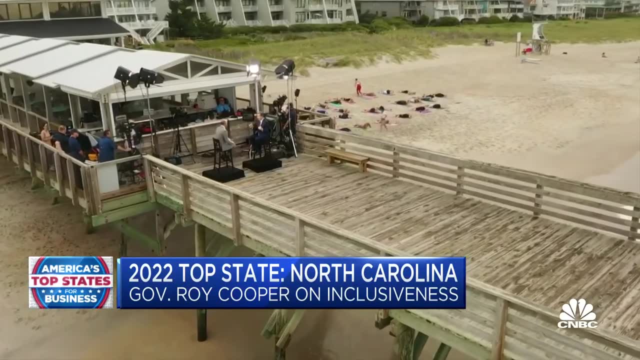 They come to Wilmington, North Carolina, just this past week in order to finish their film production, So we're sending the right kind of signals. We do need statewide anti-discrimination. I'm pushing for that. The Republican General Assembly is one of our disagreements. 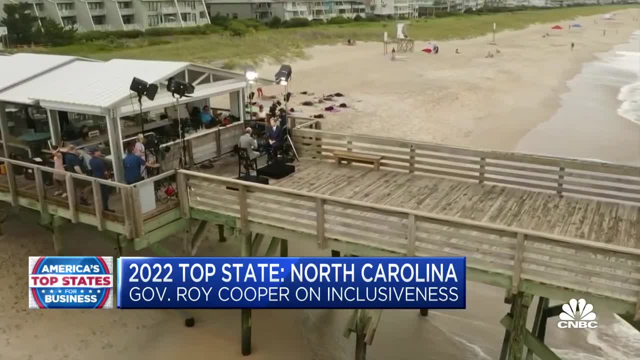 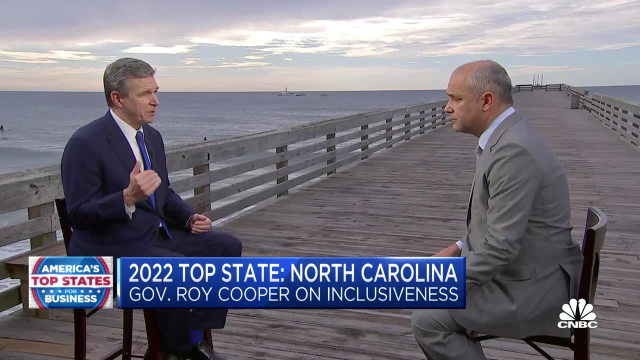 They haven't gone that far yet. You mentioned abortion. It's legal here. Will it stay legal? What do you have to do to achieve that? Well, it will as long as I'm governor, because I have vetoed bad abortion bills. 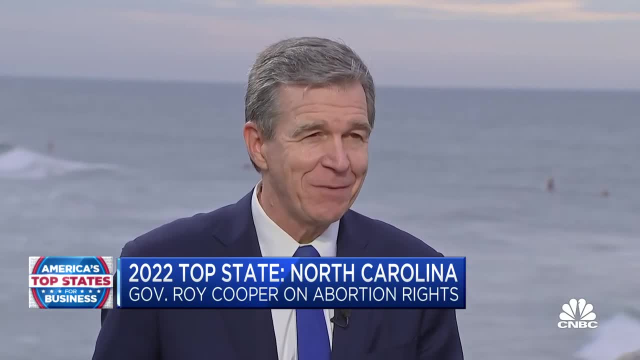 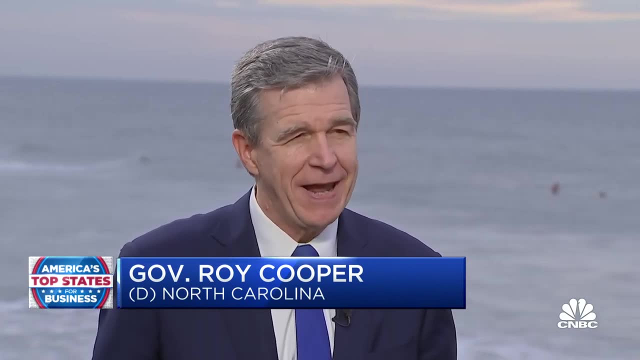 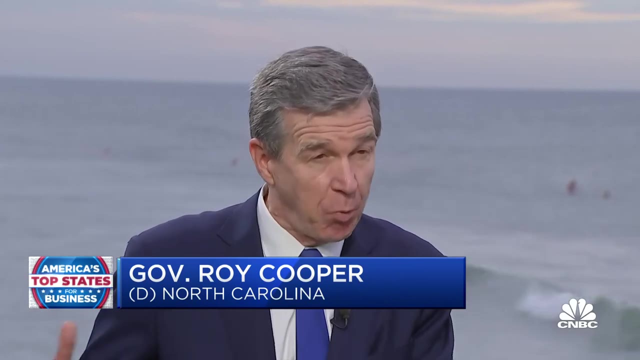 We are going to have November elections. I'm sure that I have enough Democrats in the legislature to sustain my vetoes. going forward will be important. I think we understand that I will protect women's reproductive rights. I will not back down. I think that's important for women across our state and country. 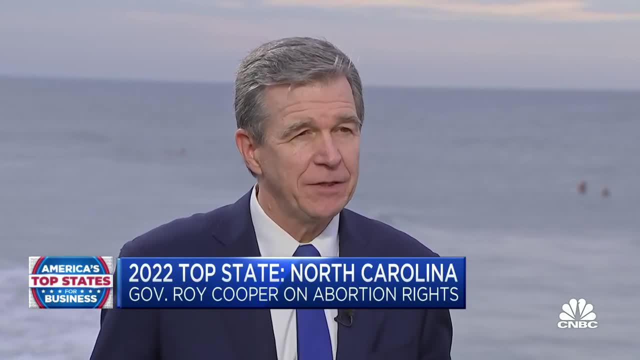 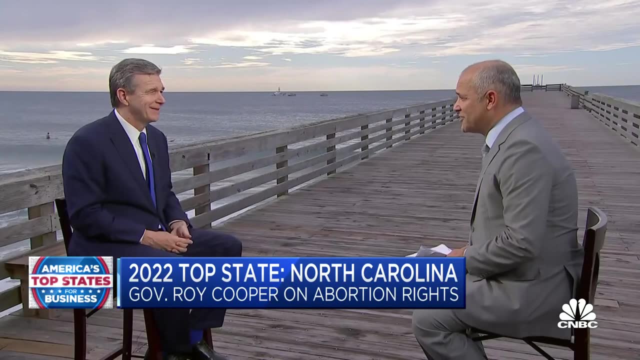 But it's also good for business. It is the right thing to do. Businesses know that they need to have their employees protected. Governor Roy Cooper, we thank you very much for being with us. Congratulations on finalizing. Thank you very much. 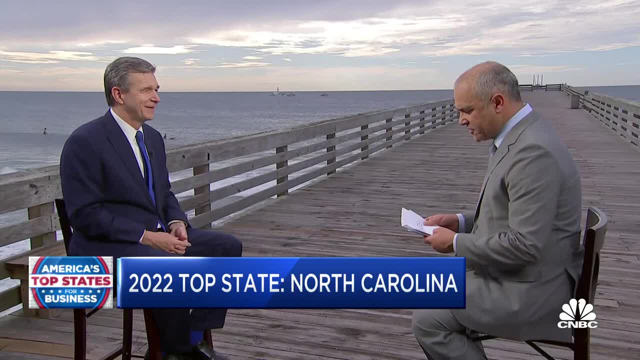 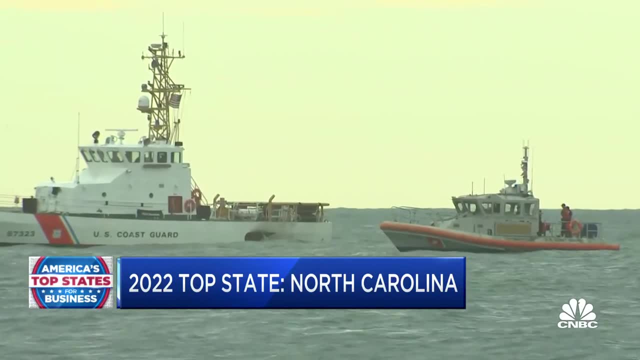 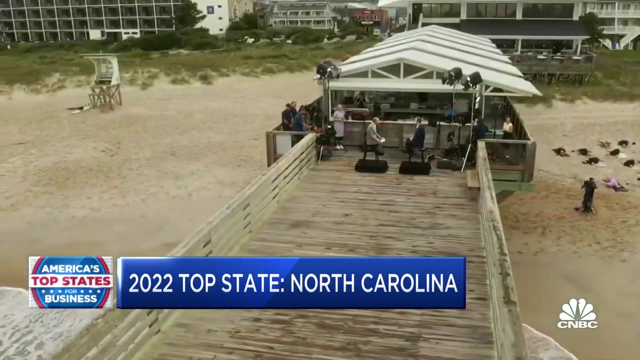 I have been thinking about the United States. This has been a very important day for the United States, especially because currently, being the top state, I think we can show we have the US Coast Guard cutter Seahawk offshore, along with a couple of responder boat mediums out of the Coast Guard Station Wrightsville Beach. 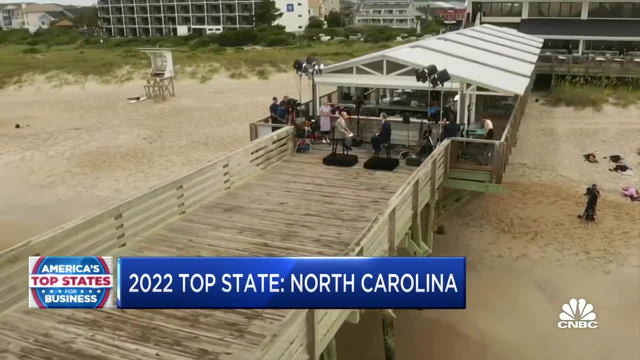 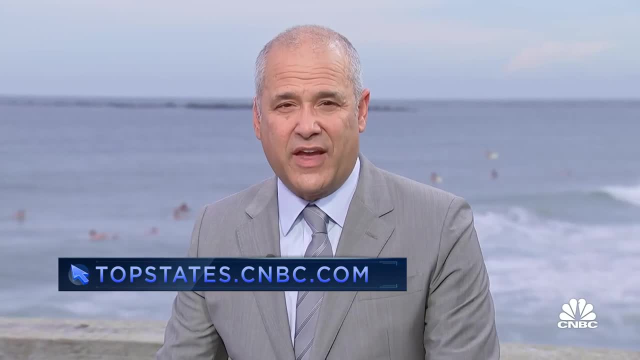 And we thank the folks at the Crystal Pier and the Oceanic Restaurant here in Wrightsville Beach, where we are live this morning. We also want to tell you that you can now see where your state ranks topstatescnbccom.